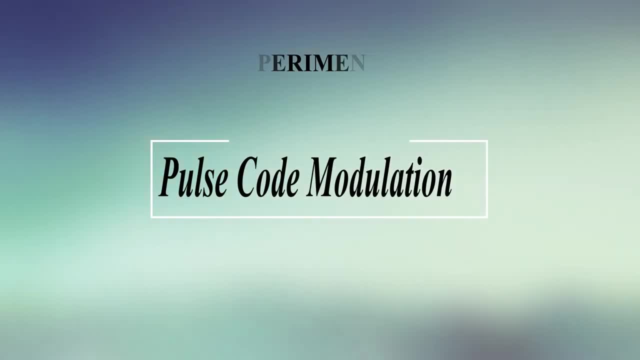 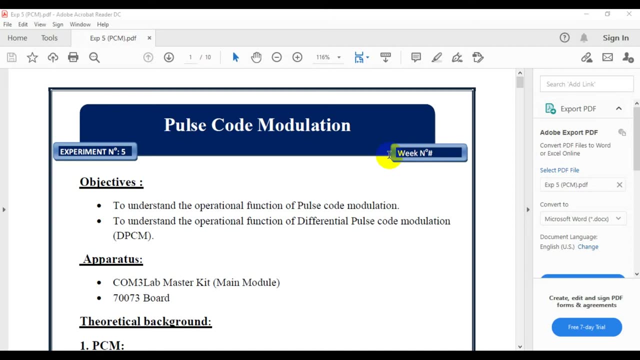 Good morning guys. Today we are going to perform experiment 5, pulse code modulation. So what is the objective of the experiment? To understand the operation function of pulse code modulation and to understand the operation function of differential pulse code modulation, DPCM. 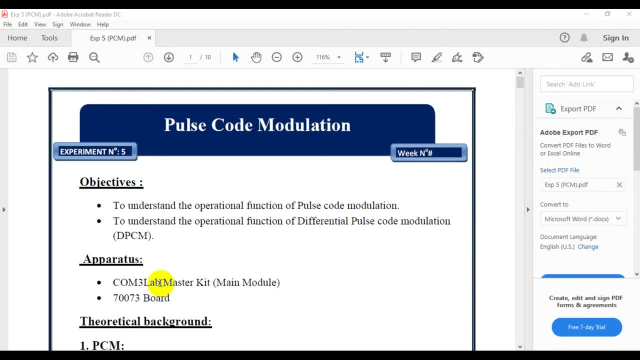 So what are the apparatus we are going to use? It's COM MasterKit Mainboard and the board we are going to use is 70073.. For the previous experiment we used 73, only For pulse amplitude modulation for the previous experiment. So now 73 board is totally digital. 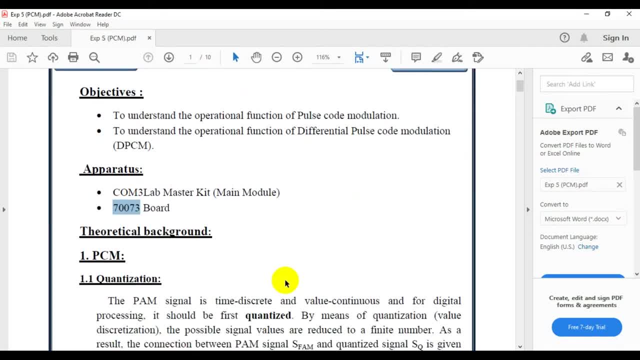 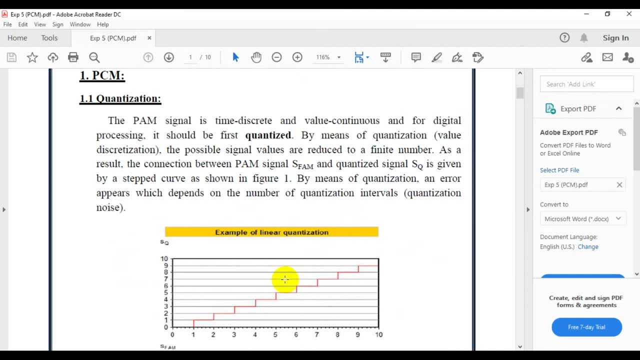 board. So DPCM comes under the digital. So what are the output we got in the pulse code, amperage, pulse, amplitude modulation. So what are the output we got in the pulse code modulation? That thing we will do, we will just sample, sorry, we will quantize it, Okay. 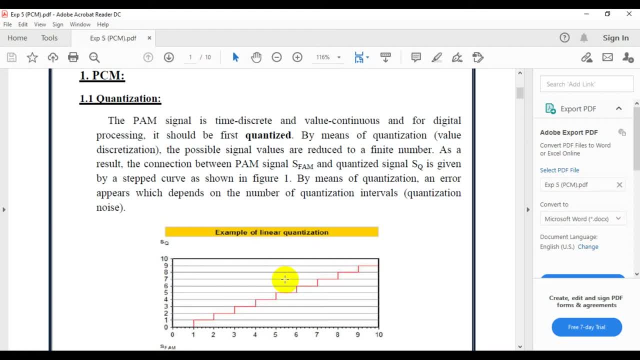 we got a sample output from the pulse amplitude modulation. Okay, After sampling we will get, we will do the quantization. So after quantizing you will get the quantize signal SQ. This is given by the step curve. Okay, Then this curve is just like a flat surface. 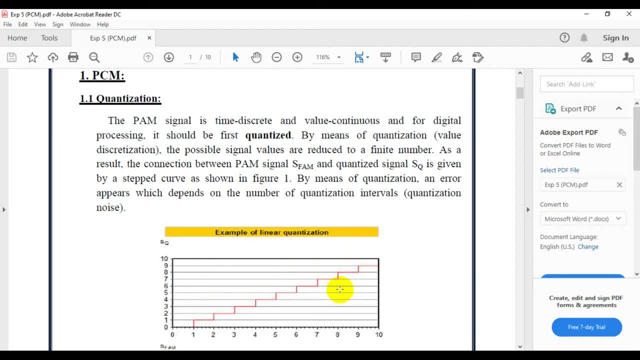 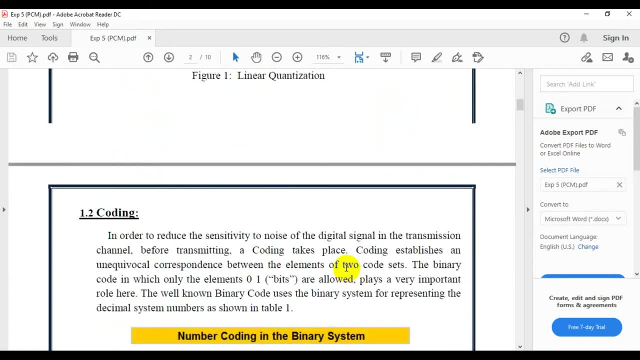 You will get the flat surface, The samples. you will make it approximately to this flat surface. This is nothing But flat top sampling like, and later we will do the coding. Okay For 0,. it is 0, 0,. 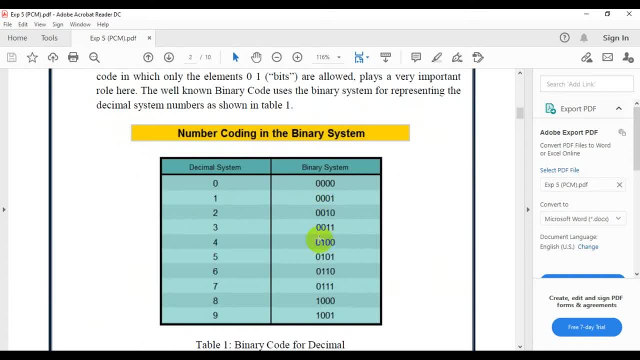 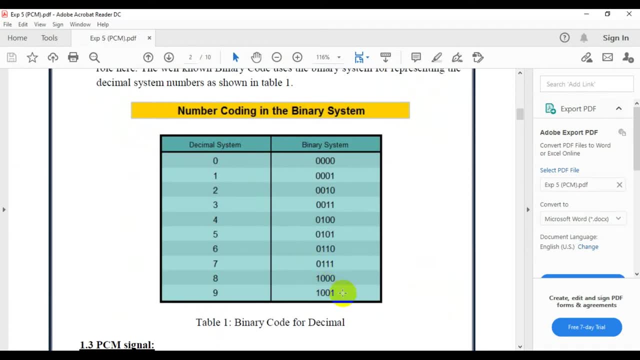 0.. For 1, it is 0, 0, 1.. 2, it is 0, 1, 0.. So on. Okay, So this is the we are. we are, this is I think we are going to perform in today's experiment. Okay, Let us start with. 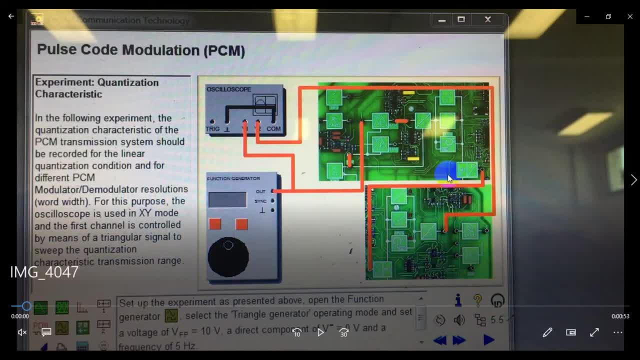 the experiment, The pulse code modulation. Okay, This is the circuit diagram to generate the pulse code modulation. So, before starting the experiment, let us start. let us start with the have the brief idea of the experiment. First, we are going to generate the pulse. 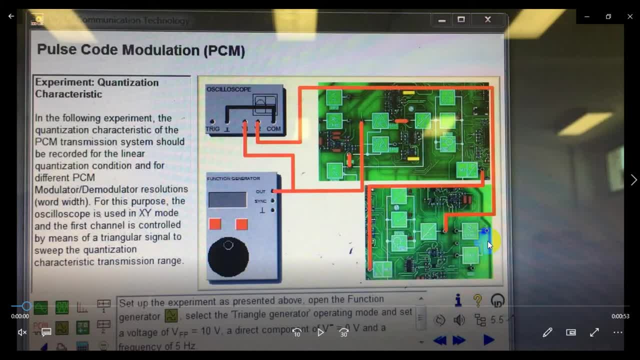 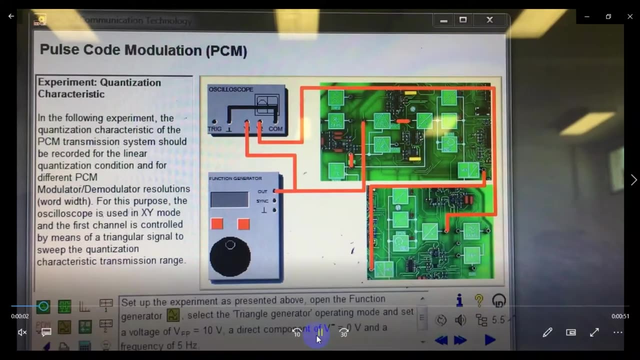 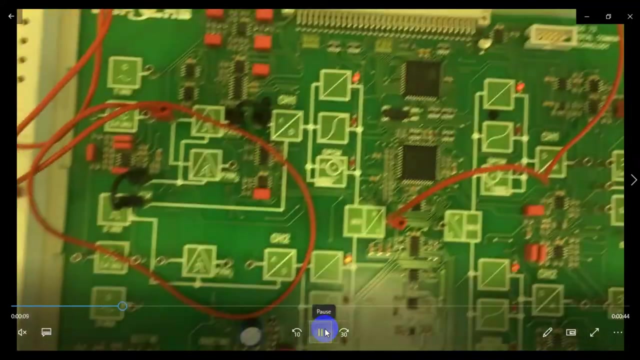 code modulated output. Okay, Depend upon the quantization step, how many quantization step we are giving, And then we will see the pulse encoded signal and then we will go to the DPCM. Okay, This is pulse code modulation, PCM. Okay, Here you can find, this is a board. 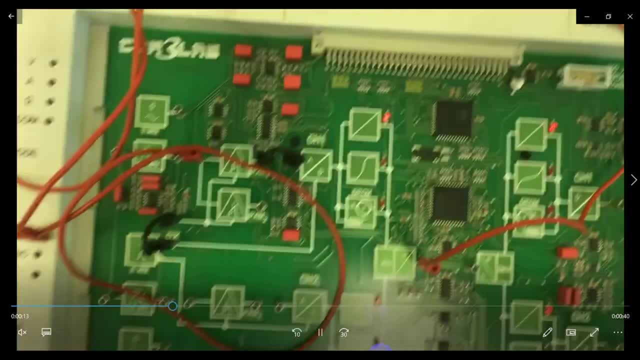 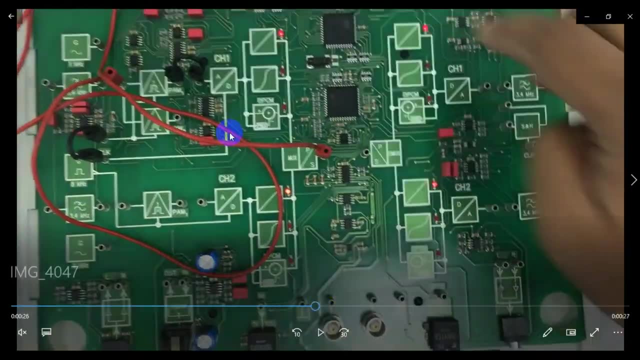 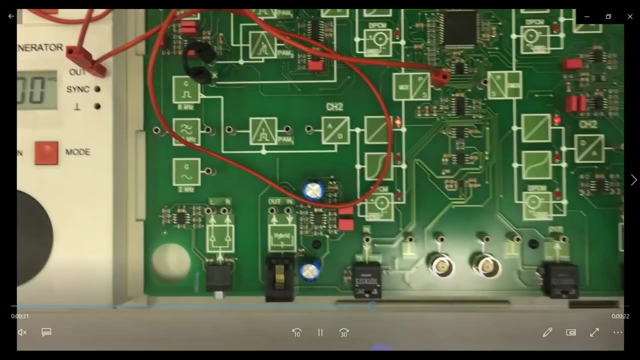 Okay, The board number is 7, 1, 0, 0, 7, 3.. It is a board number you can find here. Okay, So let me do the connection here. You can see the connection. Just verify the connection. 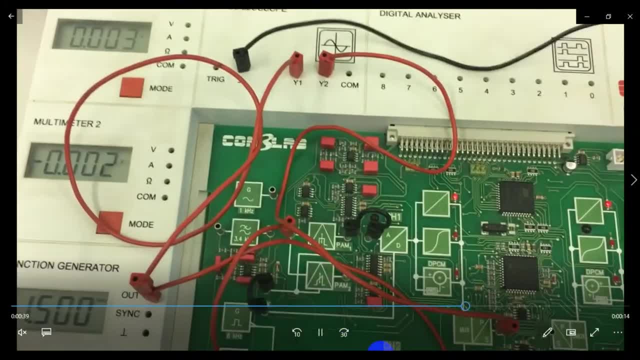 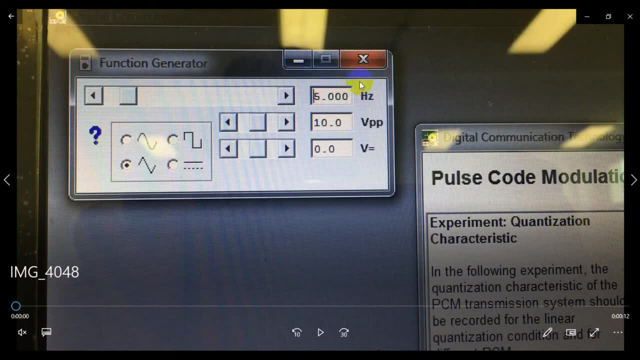 with your circuit diagram. Okay, Okay, Okay, Okay, Okay, Okay, Okay, When you go to the procedure now, just, we have to set the frequency to the four, five kilo, five Hertz, not kilo of fight hurt, And the waveform is a triangular waveform. 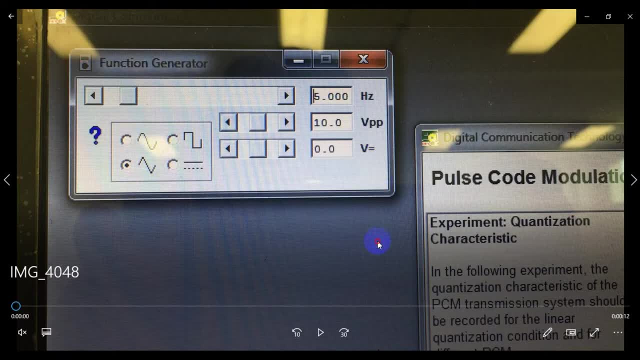 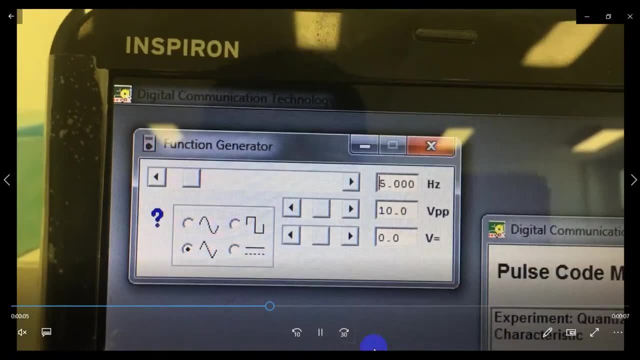 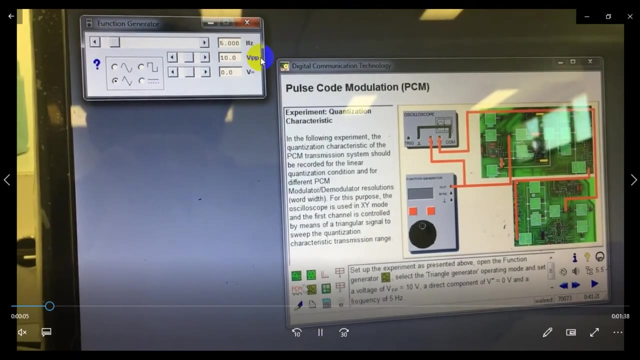 here. Okay, And the PPP is 10,, 10 VPB, the peak to peak voltage is 10.. Okay, Five, what 10 VP to peak? and DC is zero. here we are, given the function frequency in the function generator and the 10 bond peak to peak. Okayata. 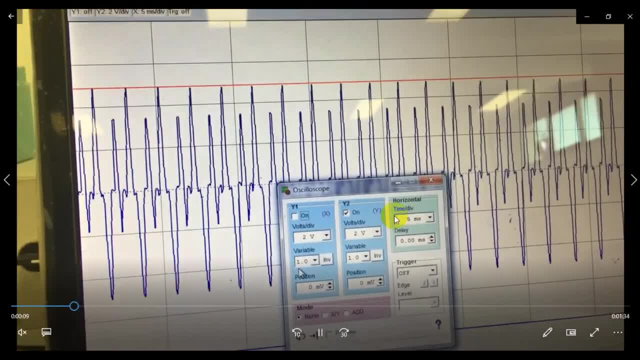 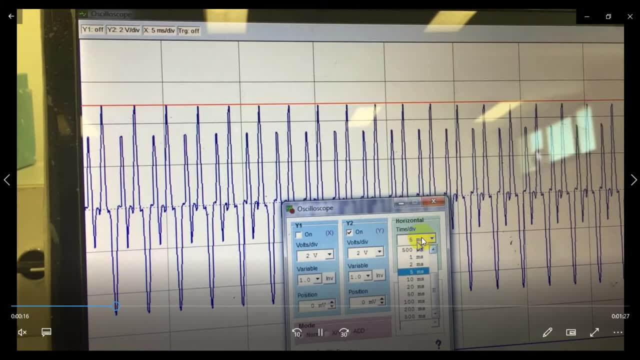 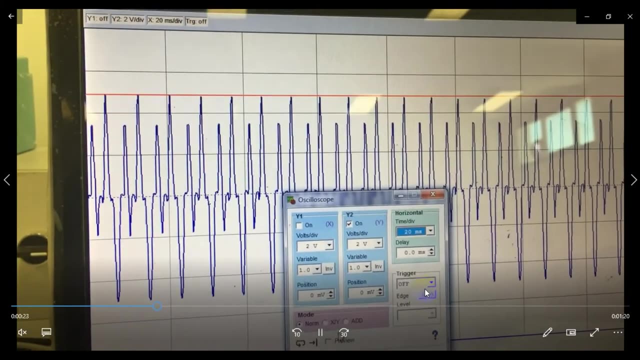 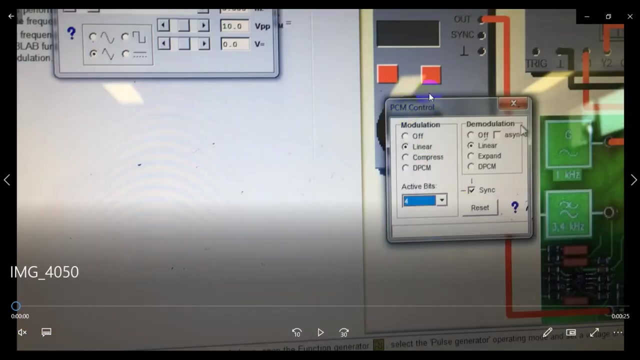 No, No, No, No, No. open the oscilloscope and say you make a channel y2 and just time per division as 20 millisecond. okay, in this case, what we are doing is where we will open the pcm control panel and we'll set the modulation into the linear form and the demodulation. okay, let me go. 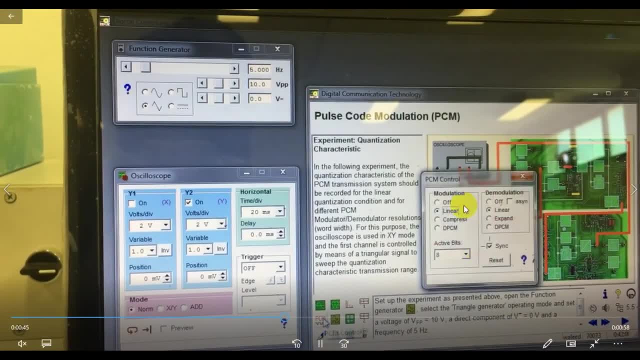 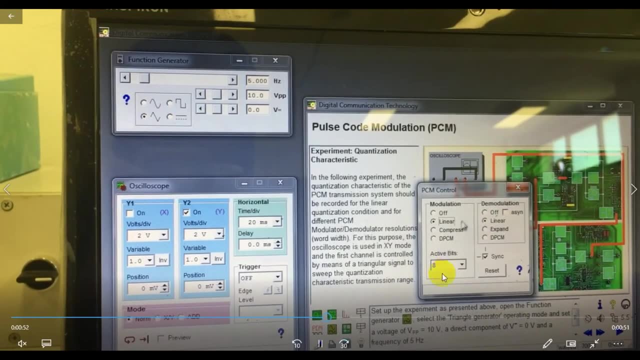 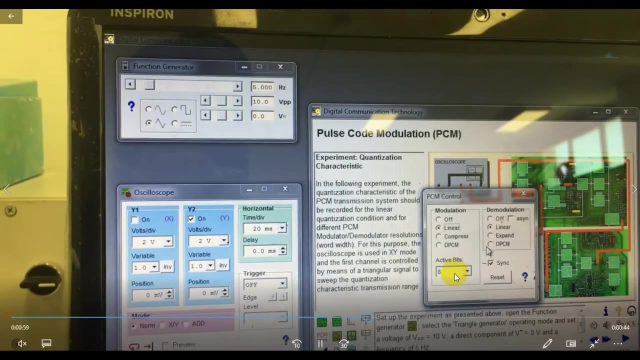 here you can find pcm control panel. okay, pcm control panel. i will set the modulation to the linear and demodulation to the linear. okay, and activates we will make it uh, depend upon the how many steps we want. okay, now the requirement for the activity is: for that mean two power four. 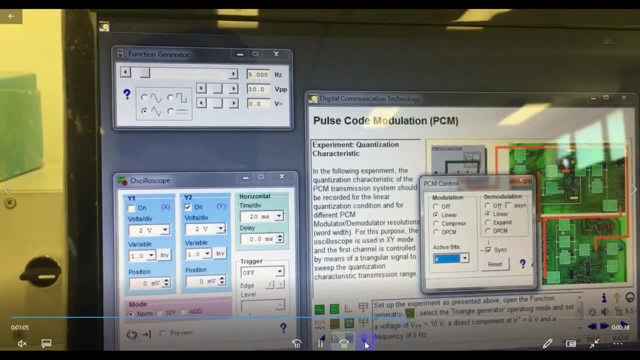 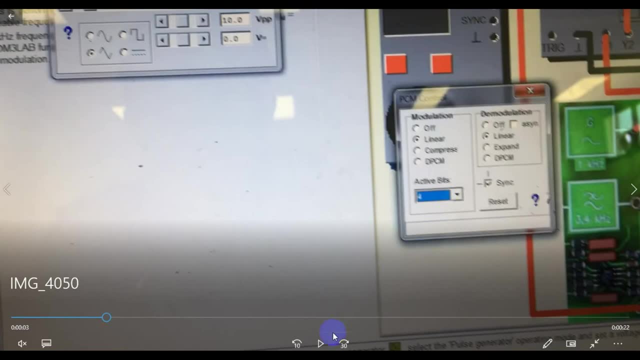 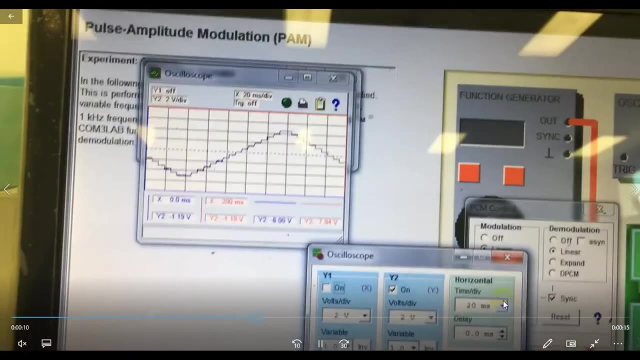 it will be two. power four is 16 step. you will get 16 steps. okay, when you, when you run this, after making two, oh sorry, four, so you will get this much steps. okay, now we have a time division as to 20 millisecond. okay, let me make it and we will count the number. 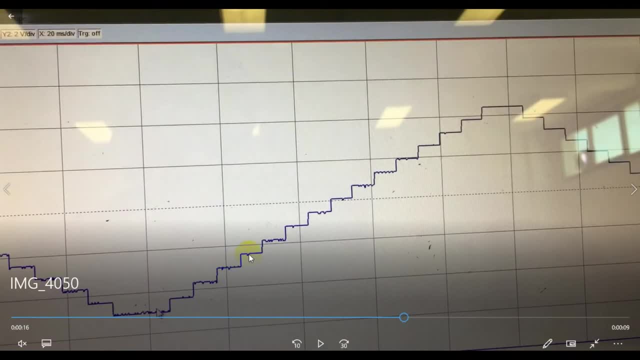 of steps here. so, if you can, one, two, three, four, five, six, seven, eight, nine, ten, eleven, twelve, thirteen, fourteen, fifteen and sixteen number of steps: that means two power four is sixteen. so, based upon number of uh bits, two power four, uh it is, it will be sixteen if it is two power five. 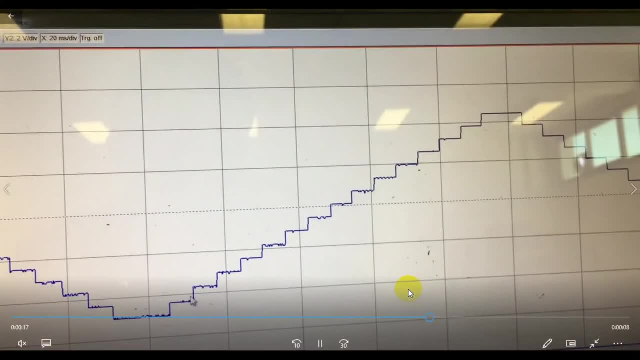 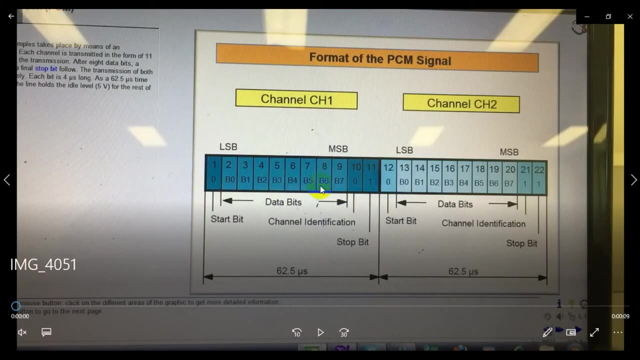 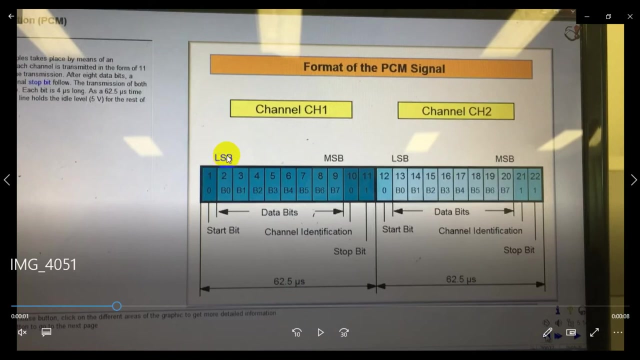 two bits. you can verify it. our next uh part is to generate pcm signal. okay, here you can see. let me show you. okay, so this is lsb, low significant bit and the most significant bit. okay, from bit two to bit ten. it were nine, it will be the data bit. okay, the b0, b1, b2, b3, b4, b5, b6, b7. okay, that means two power, three sub. 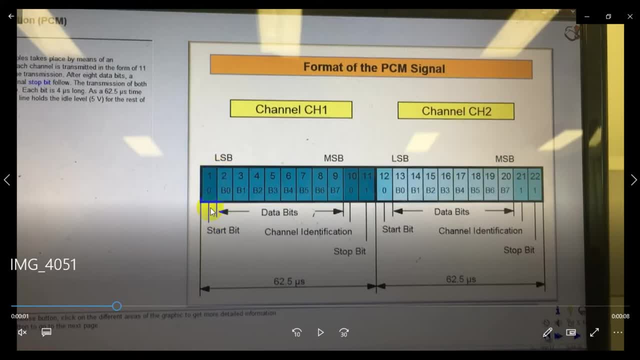 was, it is for two, power three and, and the first bit is the start bit, okay, the more lows low significant bit is the lower significant bit will be the start bit and the most significant bit will be the stop bit. okay, and the eleventh bit- sorry, tenth bit- will be the channel selection. 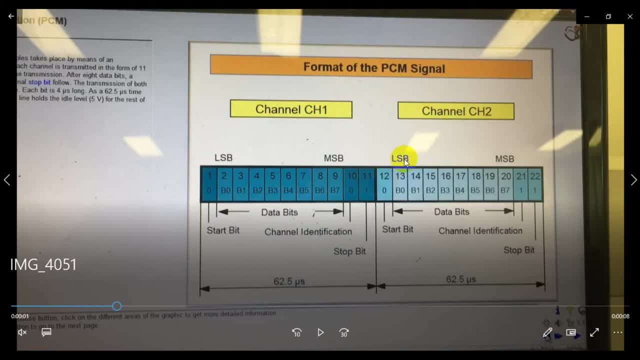 which channel you are using: channel one or channel two. so it will be based upon c. if it is zero, it is the channel one. here it is one. that means it is channel two. two, okay, so zero is here, it will be zero, and one only. so it's for zero. it is channel one we. 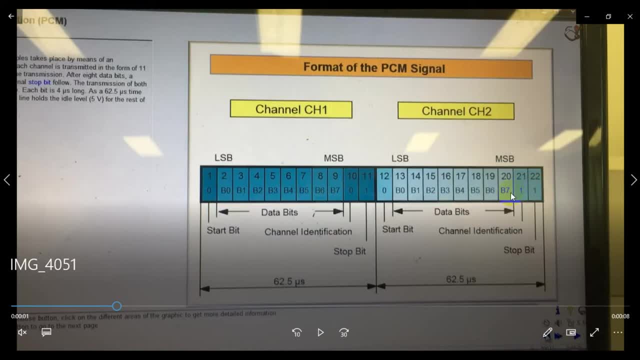 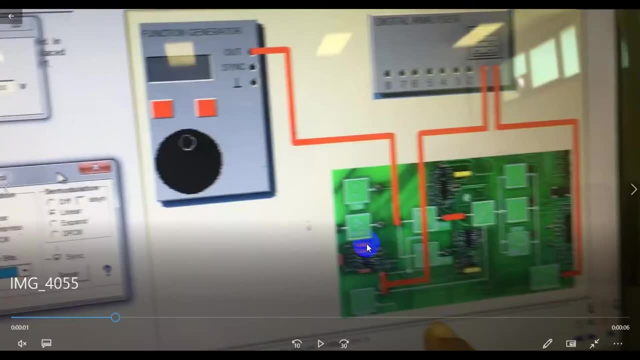 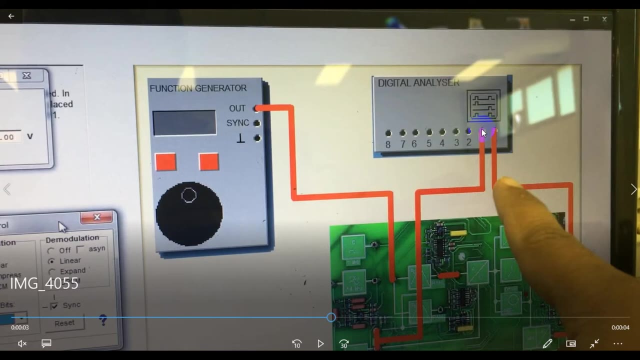 have channel two channels on the board. okay, so based upon this we will perform experiment second part. okay, so in the second part you can find only here we will connect this wire to the bit zero. okay, uh, bit zero and bit one, or we will see only the two output here. you're not taking whole. 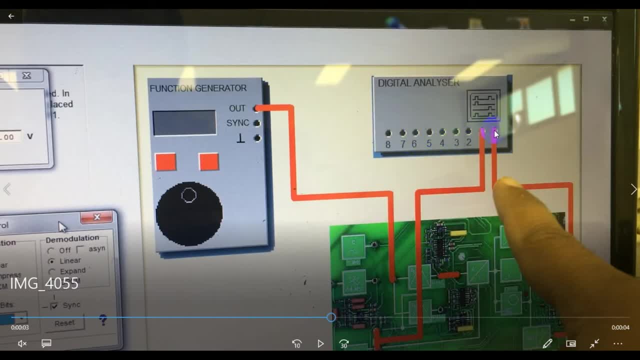 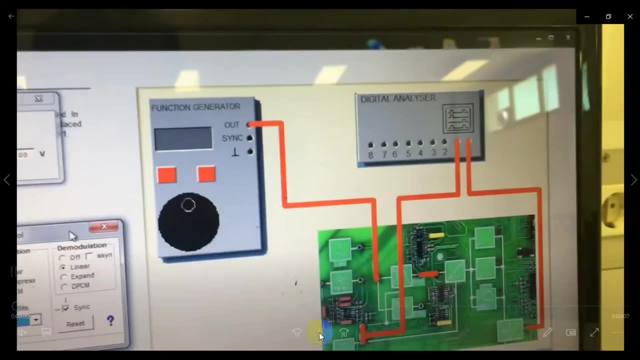 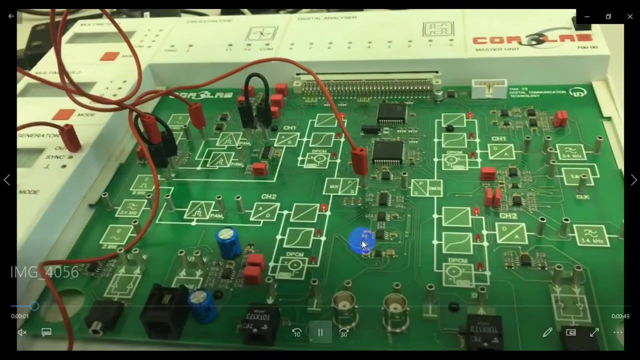 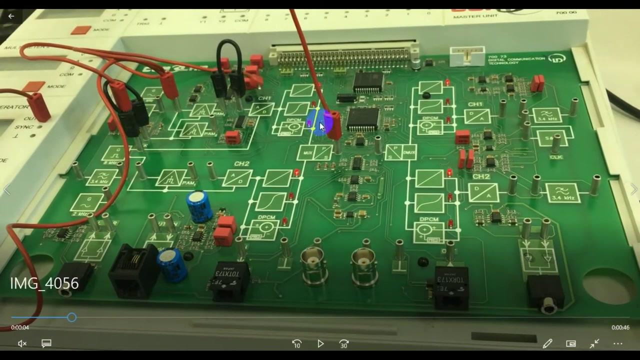 whole bits, okay, so just we will identify the zero bit, two, uh, and the one bit, only. so zero bit and one bit, okay, from eight kilohertz we'll connect it to zero and one. so here you can find. so here we'll connect this two and short it here, and this will be connected to the zero and one. 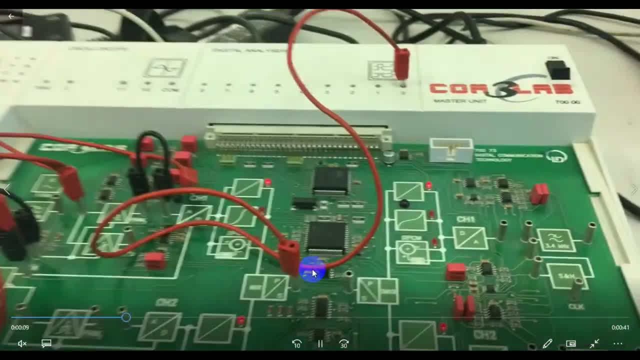 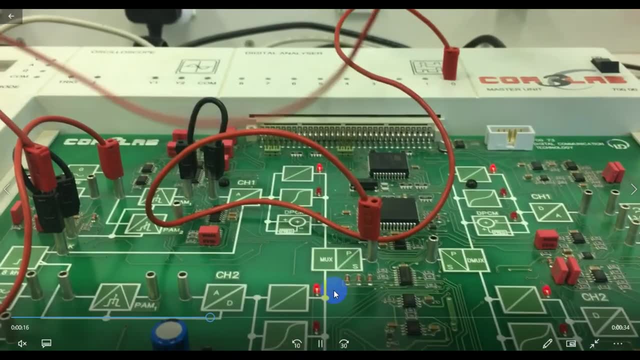 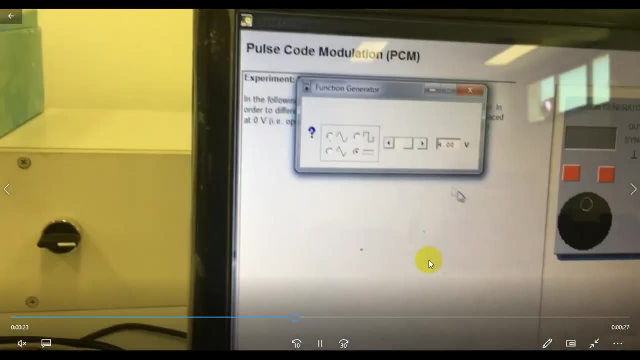 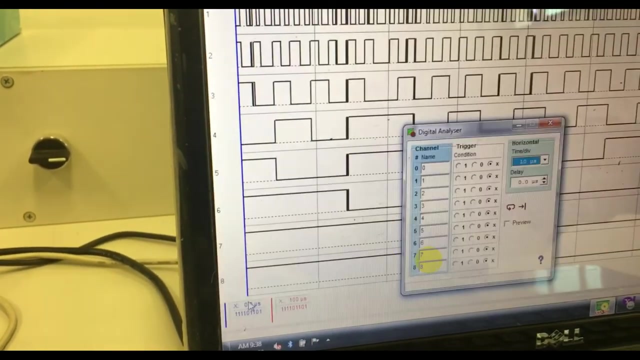 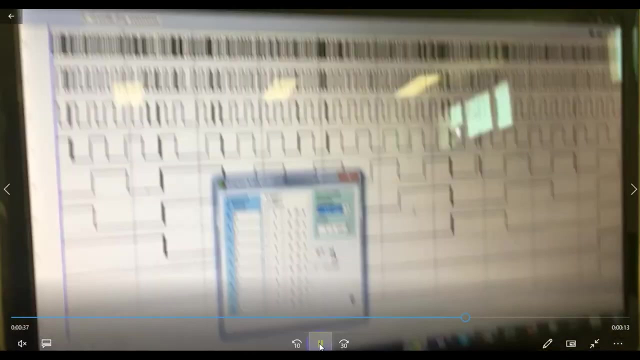 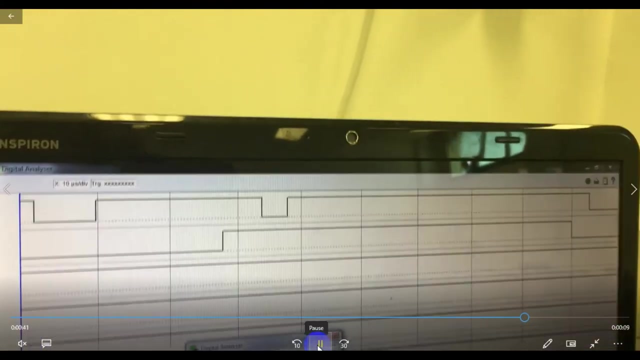 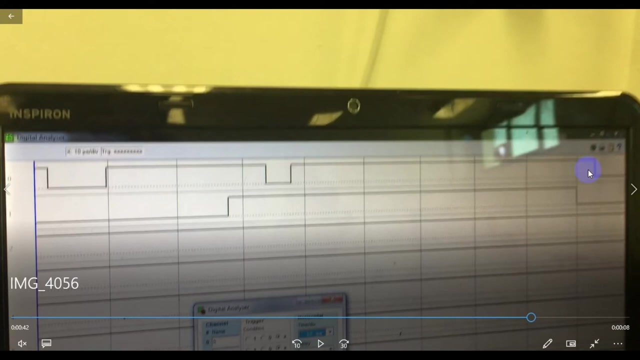 so you can see i'm connecting it to the zero. okay, from here another bit i will connect it to one. okay, then just run this. okay, now we are taking dc forward. open this digitalizer, okay. __ one, one, one. one. one, one, two, two, three, six, seven. 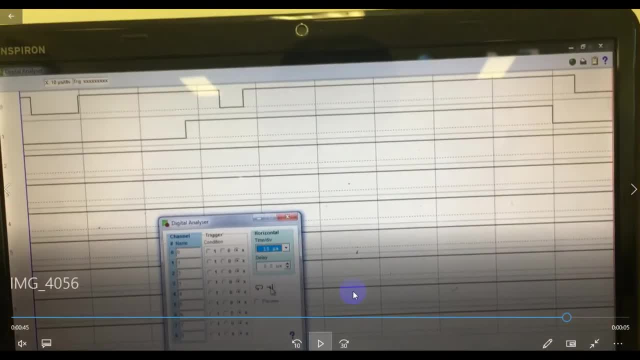 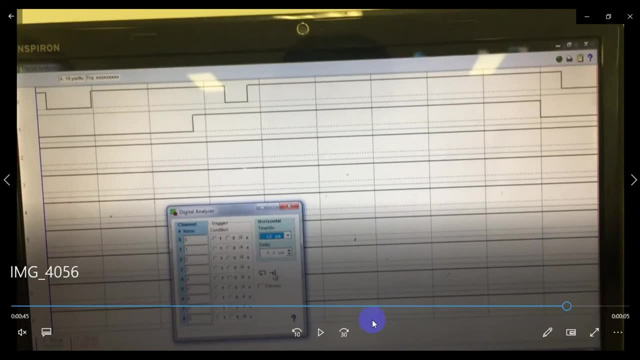 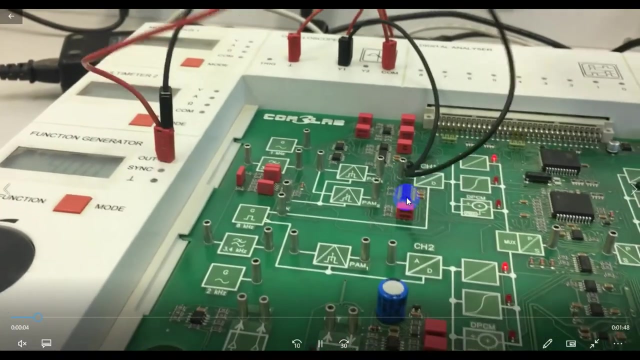 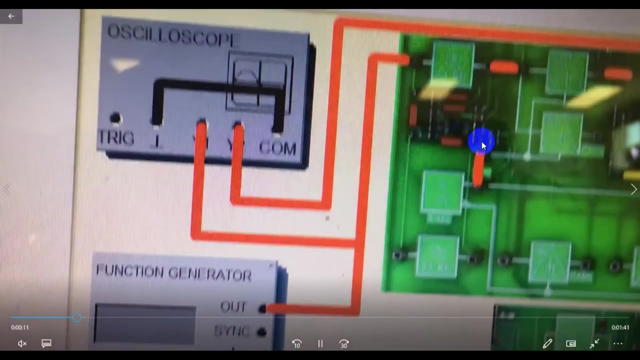 eight. so other way it is b0. it is not shown here. okay, you can draw, just simple way. this is randomly generated, okay, only generated signal. you can draw it last star, dpcm. okay, so just let us make the connection from them. just see the circuit diagram simultaneously, okay, from eight hertz to the pam. 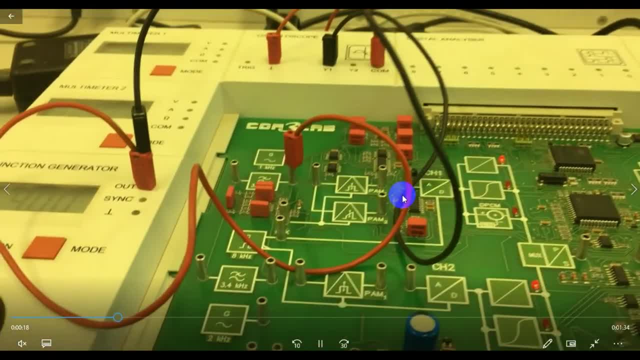 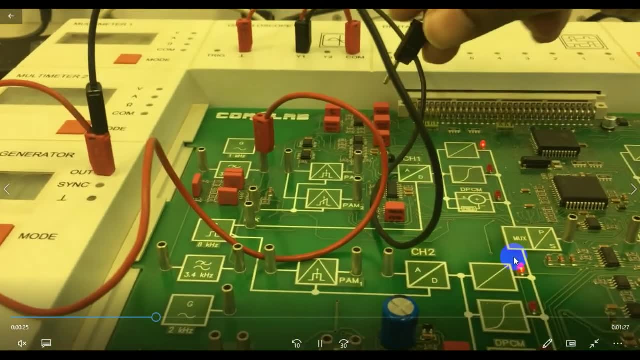 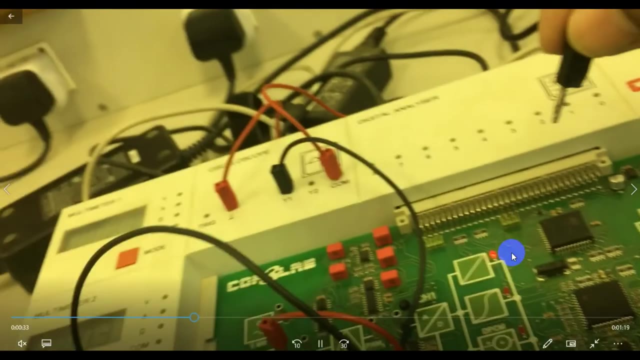 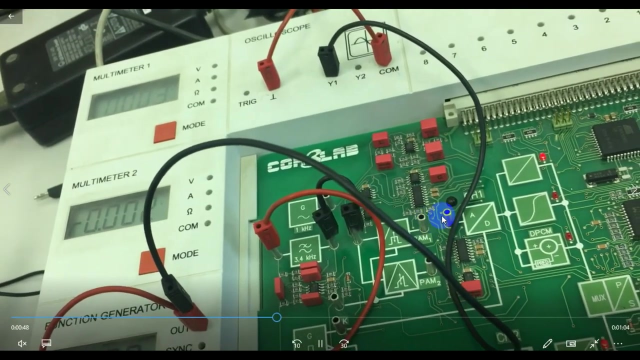 to: okay, and these two shot this. these two will be shot here. this will be connected here and these two will be short. this two will be short and this two will be short. yeah, I'm gonna get here, and this to short next to will be shorted. 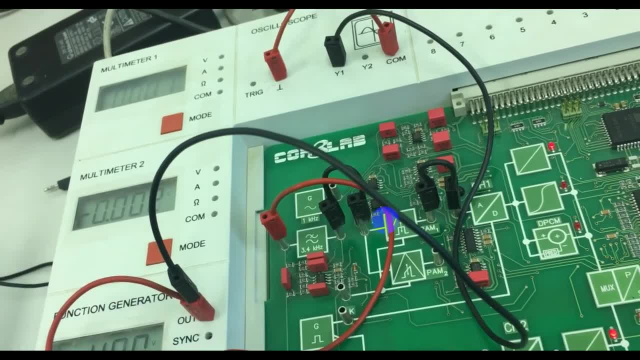 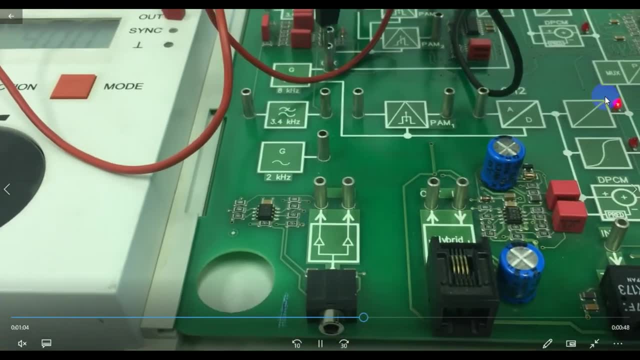 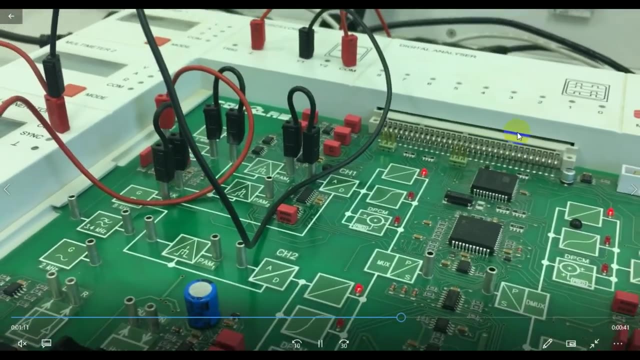 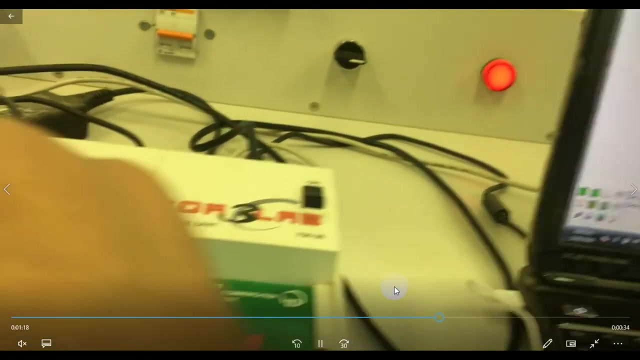 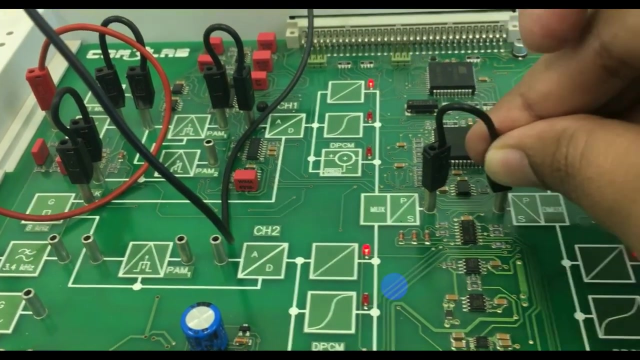 okay, then this marks to D marks. okay, first we will connect from Jeff from generator to the time to. okay, then peel palettes. parallel to series to series to parallel this one, this is serious to follow. parallel to series. okay, panel to series has to parallel. then see, here you can find channel 1 and channel 2. so here we. 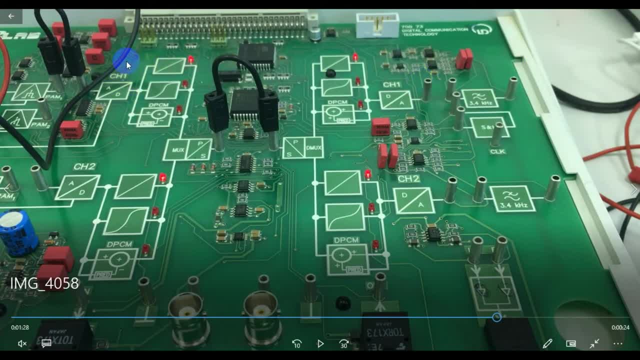 are using channel 1 here. we are using channel 1 here. we have to use channel 1 only. you cannot connect channel 1 and channel 2. you will not get the output. okay, so you are you. if we are using channel 2, then you have to connect to the channel 2 so that what we have seen in the previous signal 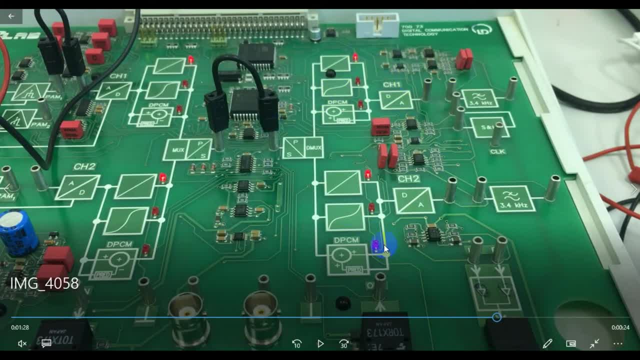 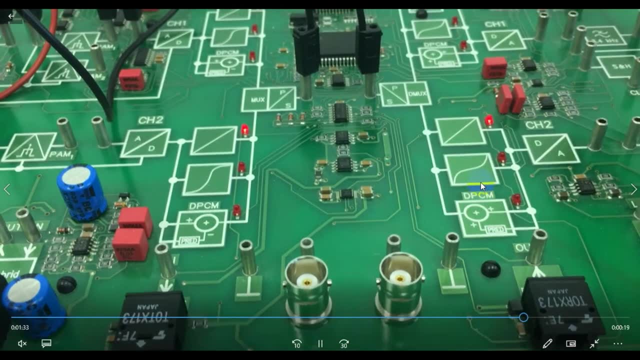 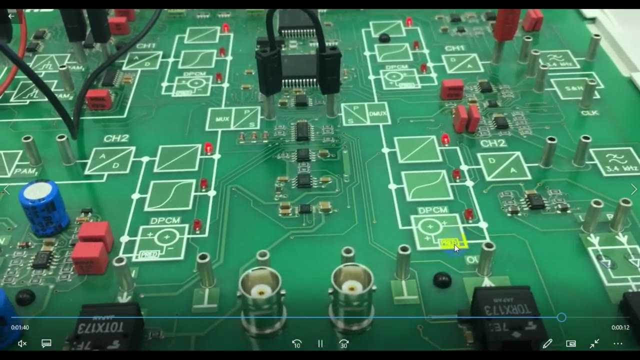 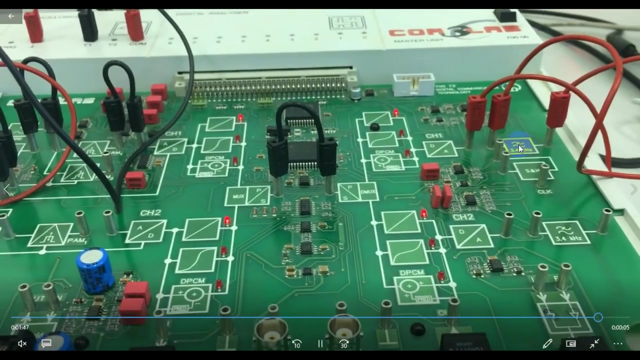 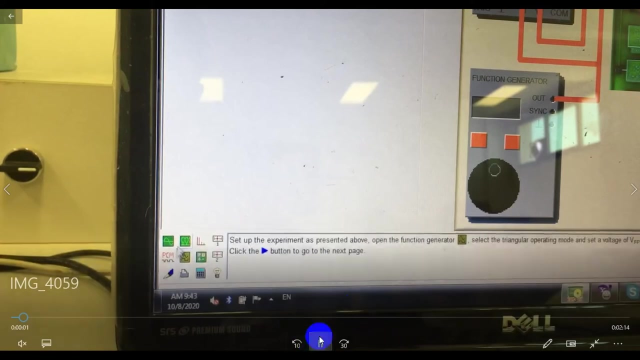 signal generation. so it was 0 for channel 1 selection and 1 for the channel 2 selection. okay, So this is the channel 1 and channel 2, okay, channel 1: digital to analog converter. okay, and 3.4. we are getting that differentiated pulse chord modulation output. so this is: 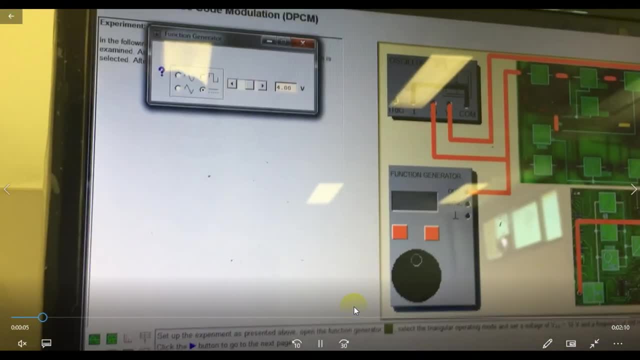 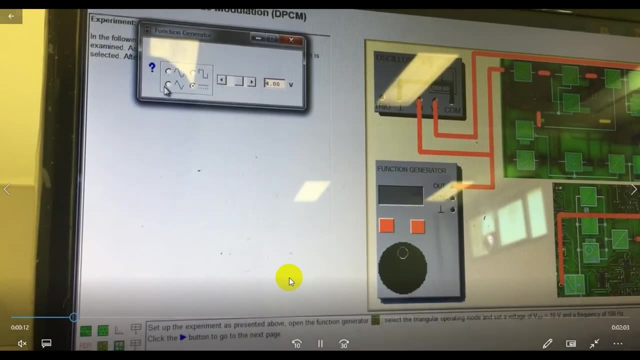 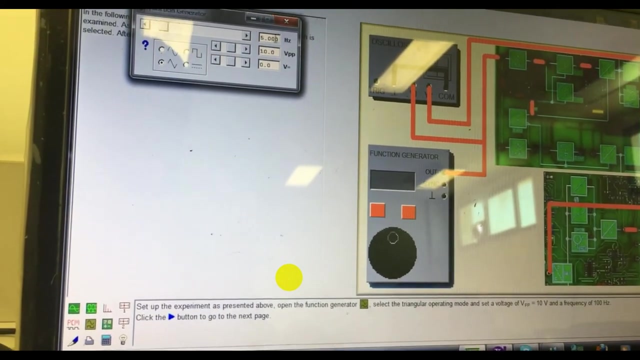 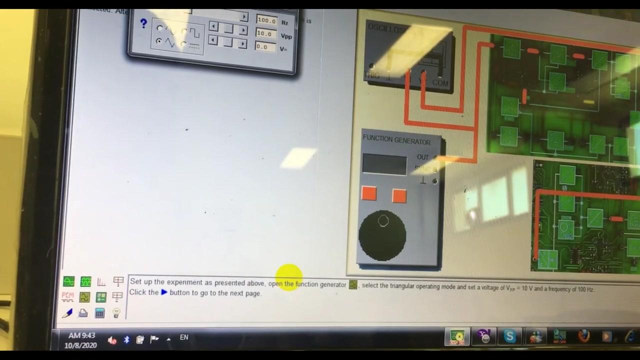 we will open the function generator and set the. set it at a triangular- triangular, okay. and make it 10 V peak to peak and 100 Hz frequency. 100 Hz frequency and 10 V peak to peak: okay, we set the function generator frequency. 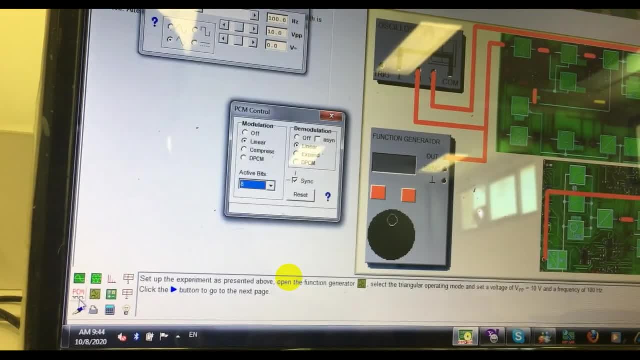 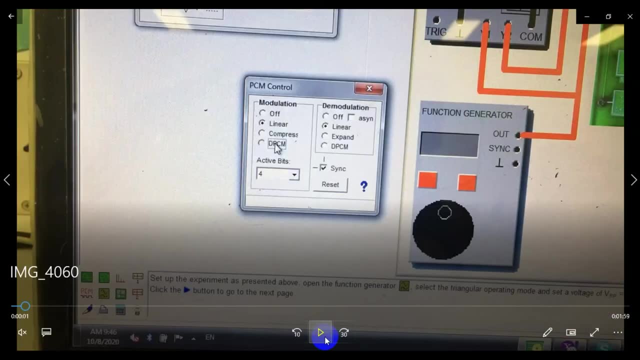 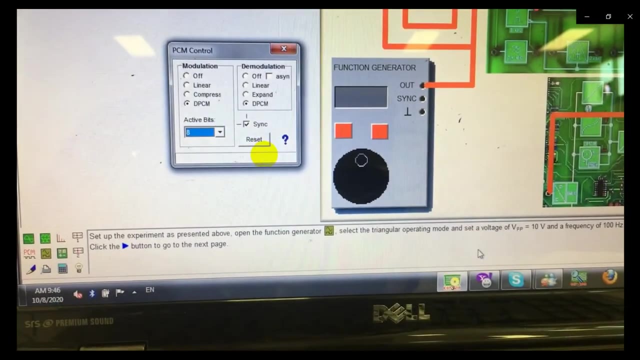 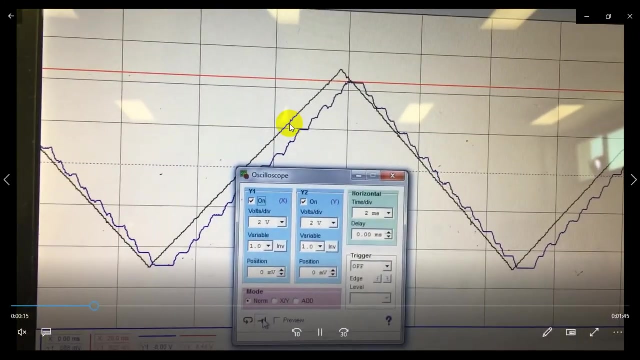 frequency is already set now and we will go to the PCM control panel and we will set it to the DPCM. okay, now we will set it to DPCM active bit as 8, 8 active bit and just take a single shot. take a single shot, okay, you will get it as okay. this is the for 8.